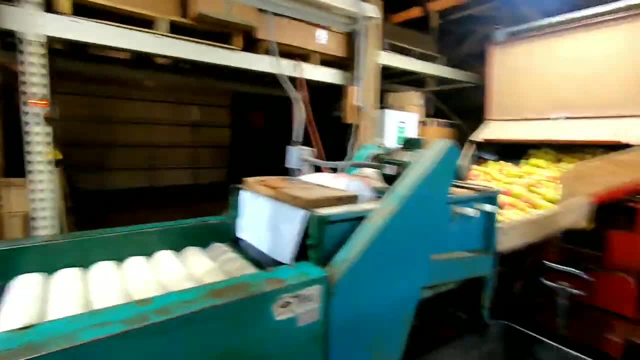 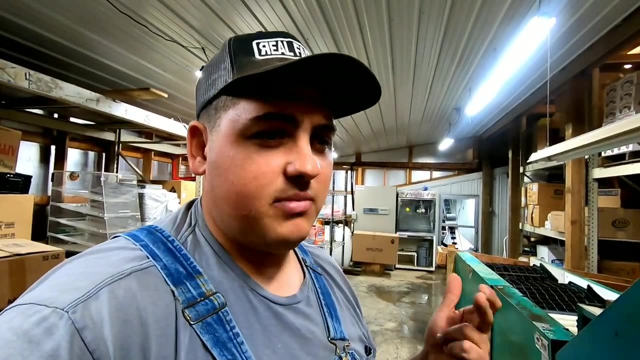 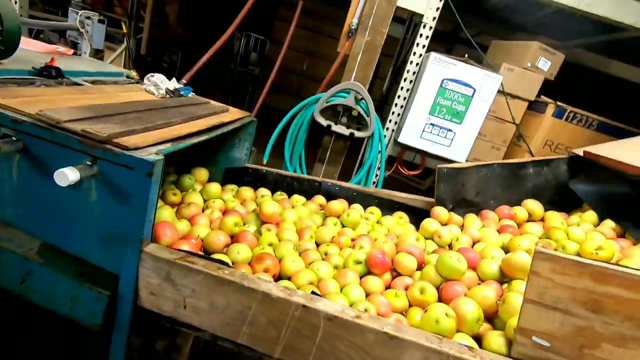 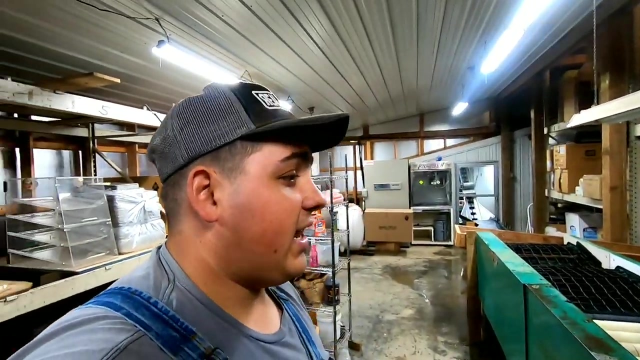 So I believe Isaac got everything cleaned out here. So he's got some Fuji's pressing these first here and we're pressing four bins and I've got Fuji's. I leave one or two bins of Fuji's, a Jonathan, maybe two Jonathan's. I got a don't even know what we're pressing, but I know we have a Red Delicious that we're going to press and then it'll be over. So either one or two Fuji, one or two of Jonathan's and then we have Red Delicious We got to press and that will be one of our last bins of Red Delicious for the season. We still got quite a bit of Jonathan's and Fuji's. 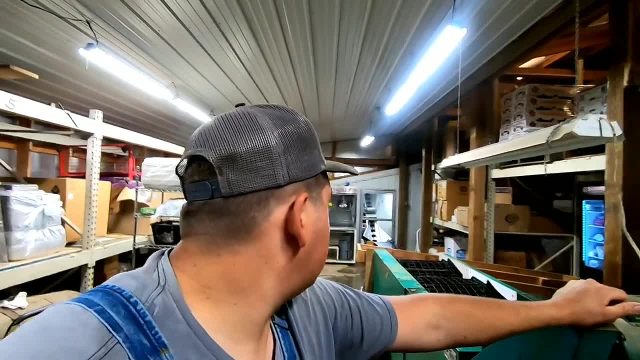 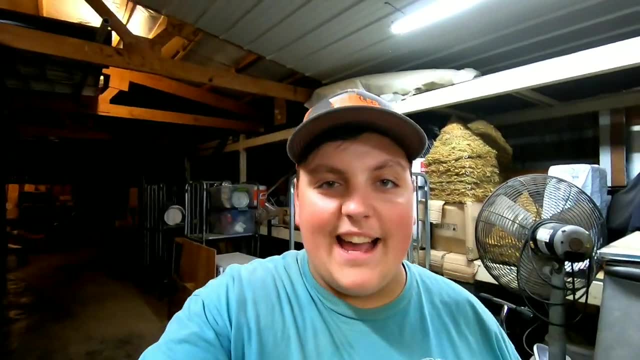 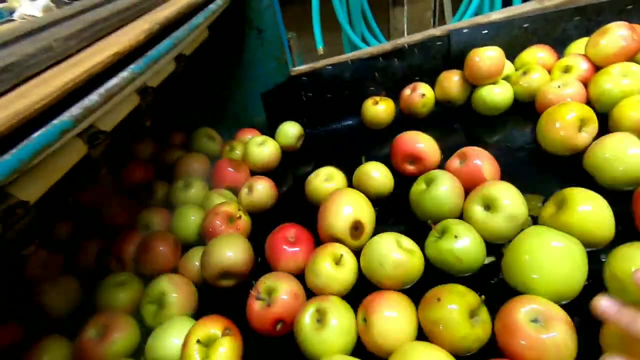 And some Golden Delicious. We've got to press into cider, but slowly and surely we're going to get it done. So, as you guys know, just stay along for the ride and we'll get it done. Hey everybody, it's Isaac and we're making cider, and my job back here is always pushing product through apples and then find a bad one like that. That is no good. 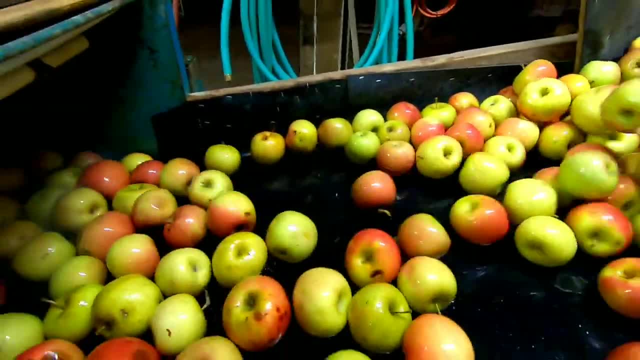 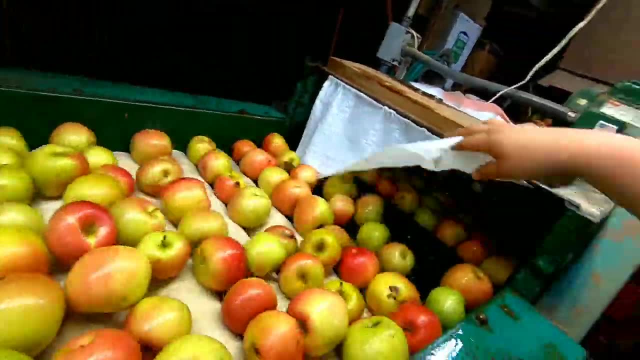 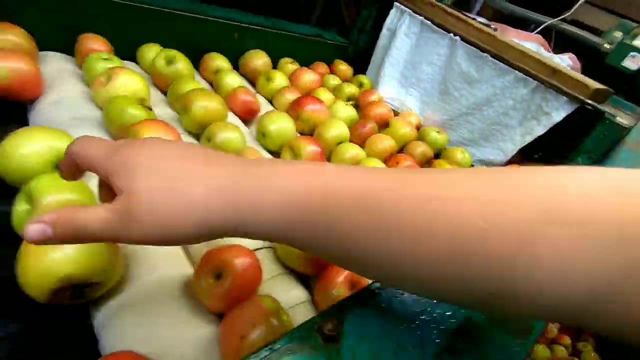 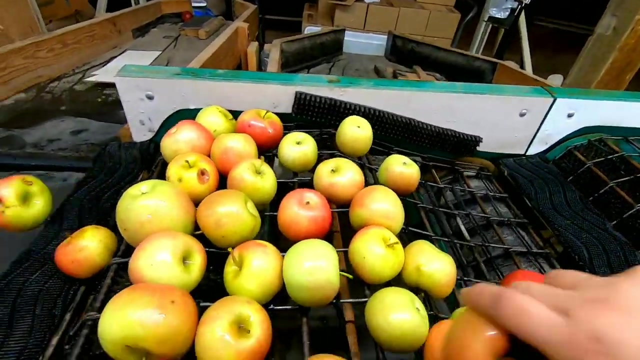 I'm just pushing, checking, See them. See there, they're coming through. I have the washer there. See, I see something bad like that right there. No good, There it is. It's coming down, this thing right here. 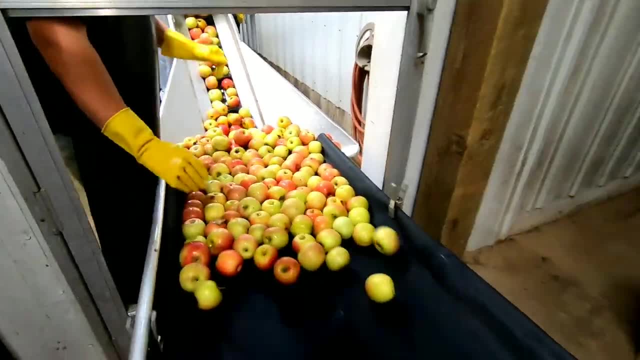 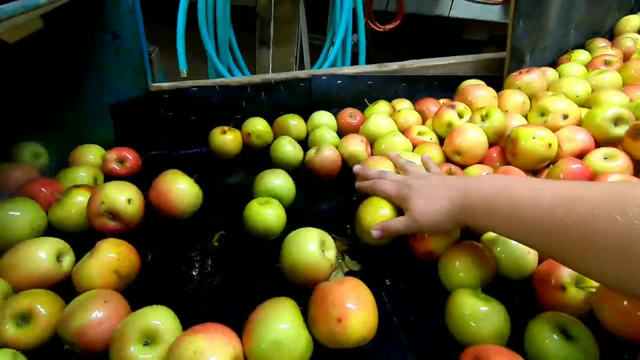 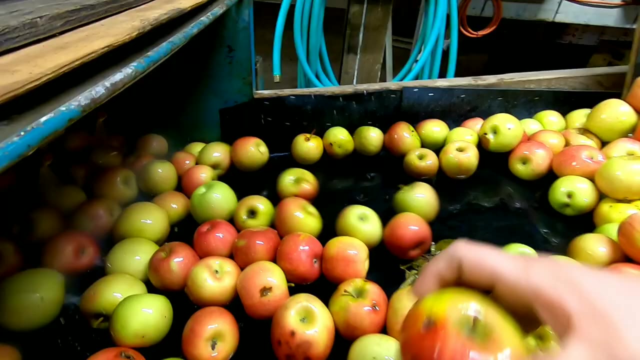 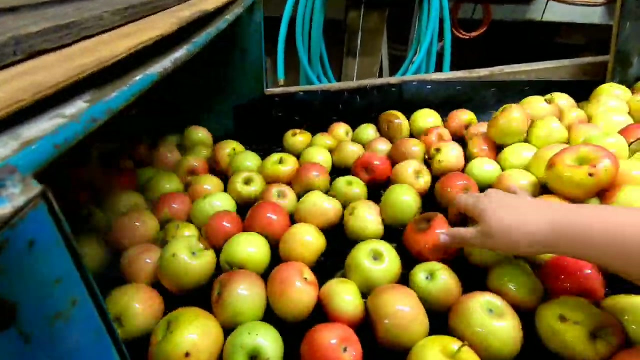 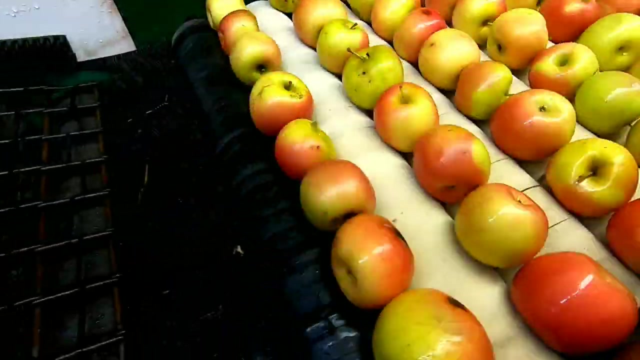 And this Here it is: Yeah, So set it right there. Arr, You don't need to cut off in there. Take it easy, brother. Take it easy on it. Yeah, There we go. So this is actually going to be a place where we can tie this. 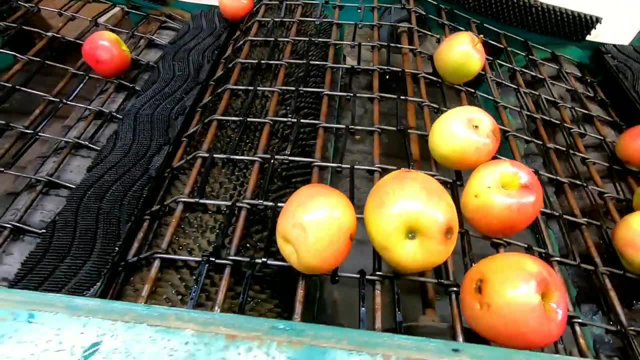 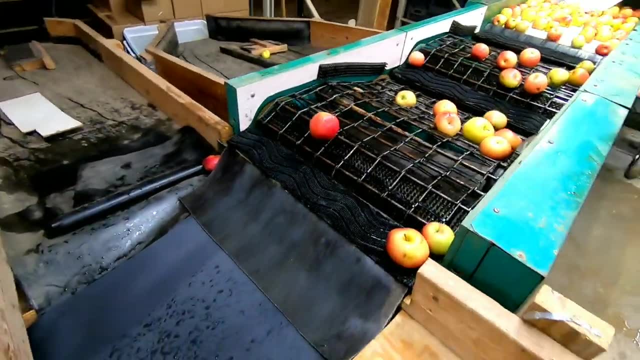 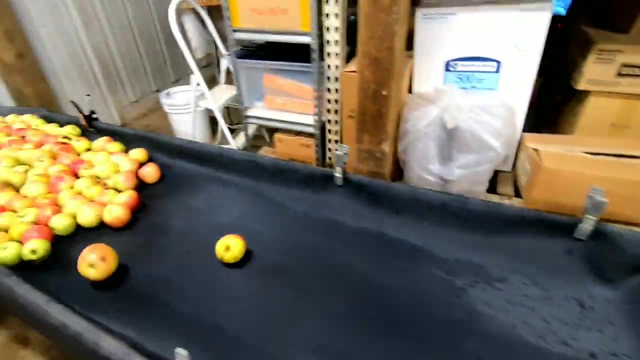 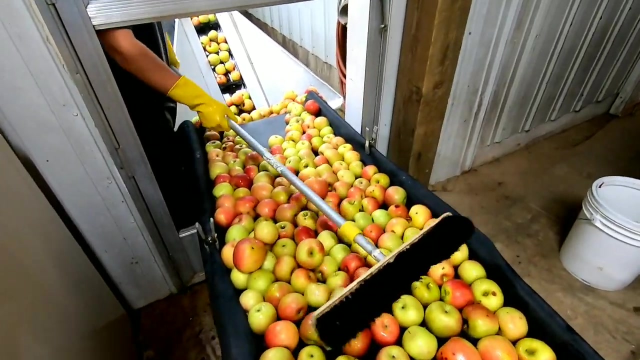 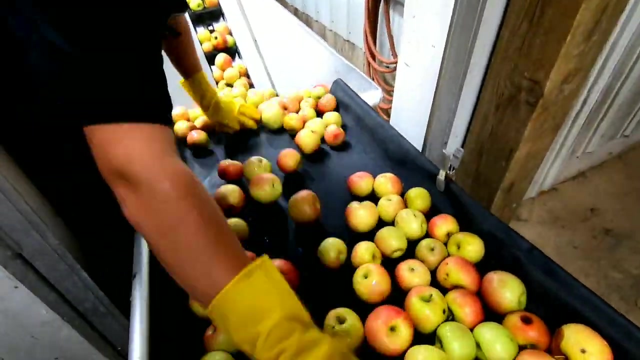 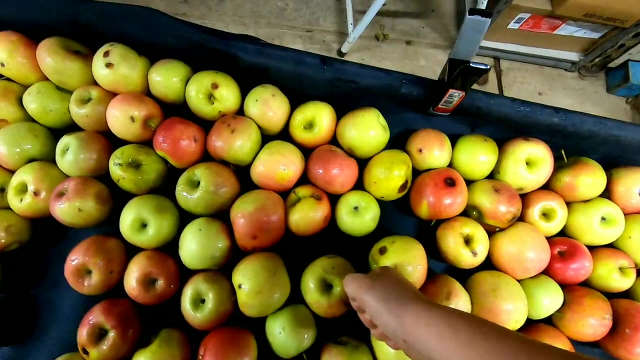 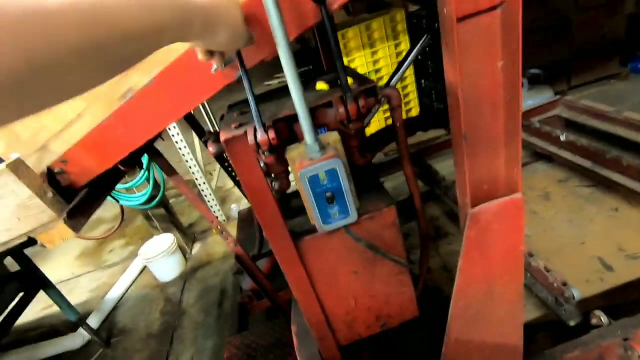 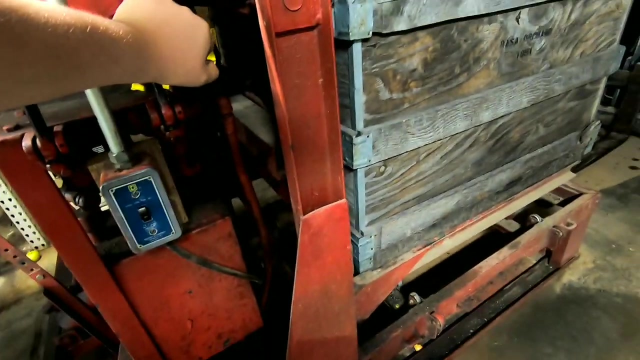 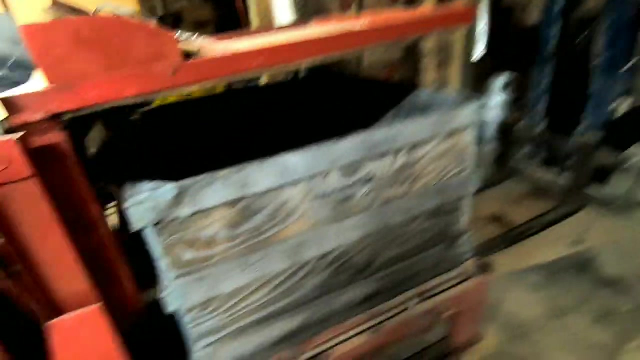 I don't know. So after the sucker's done up here, we just put the sucker down. It's a little fancy. It's my style of drawing. I come to the full limit. Grab the movement box out here. Put one of the baffles up here. 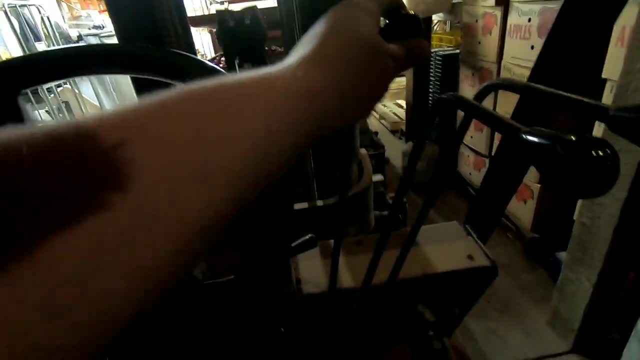 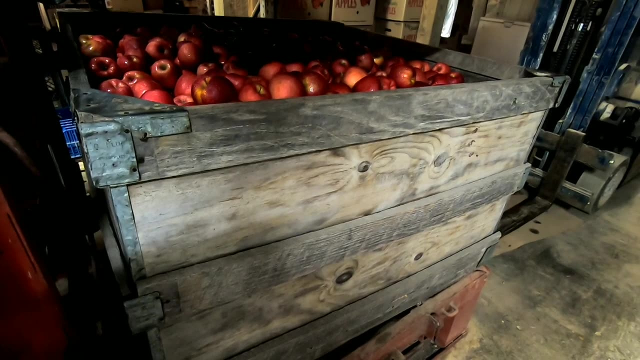 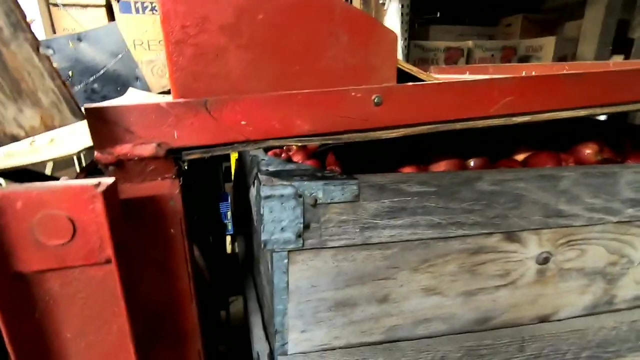 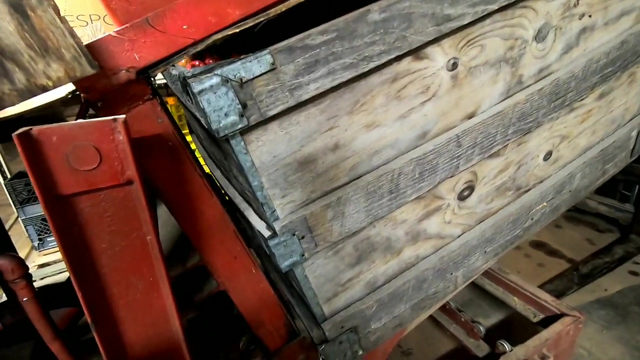 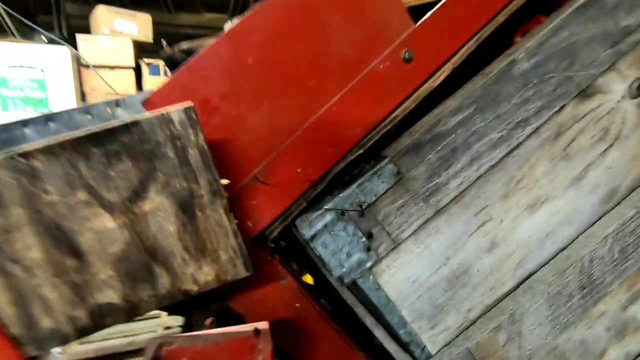 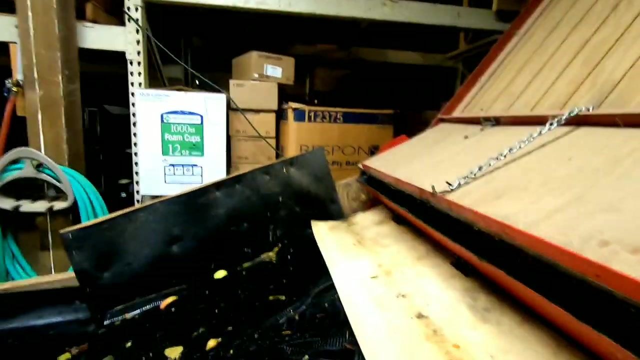 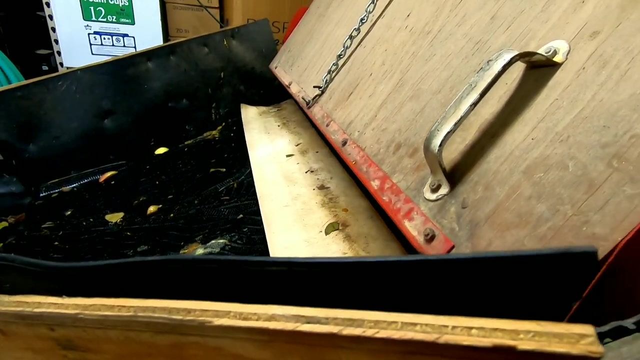 Right Yep Point at the bottom of my grass there, Pull her up There, There, There, There, There, Pressure, Pressure. sorry, That's good, And you are. I can't do this two handed, so I'll hold up here. 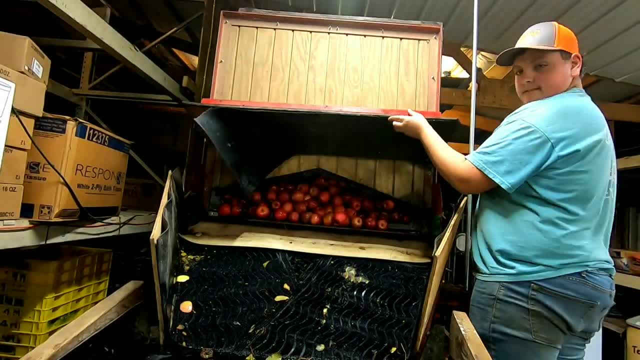 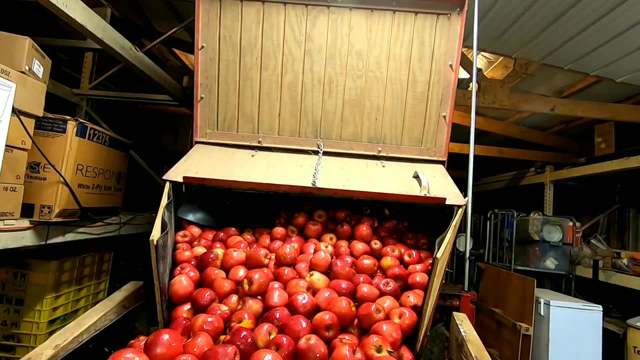 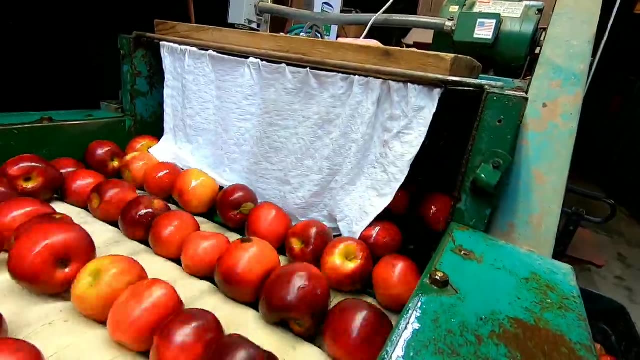 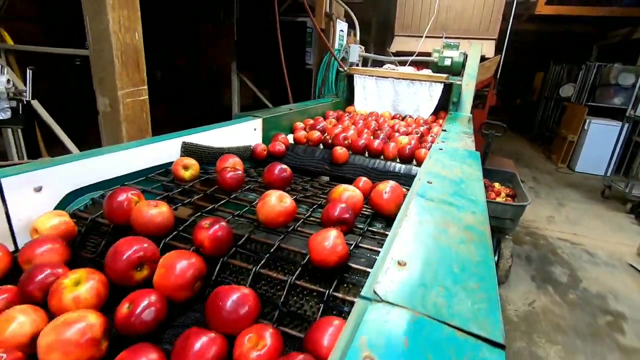 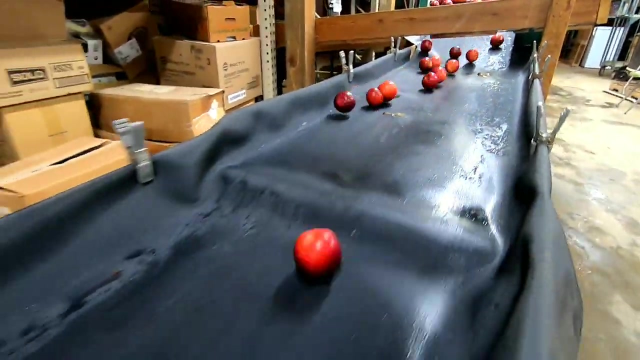 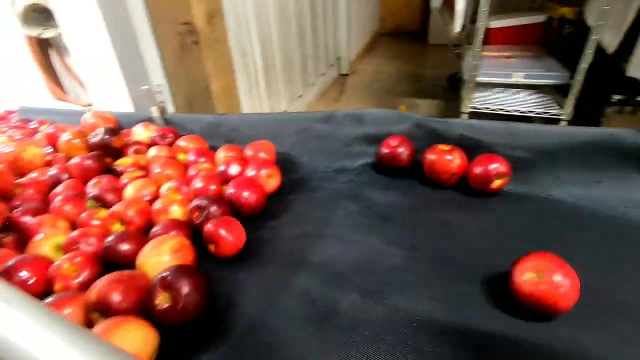 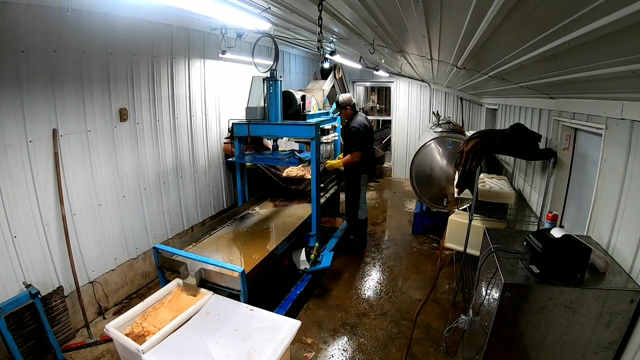 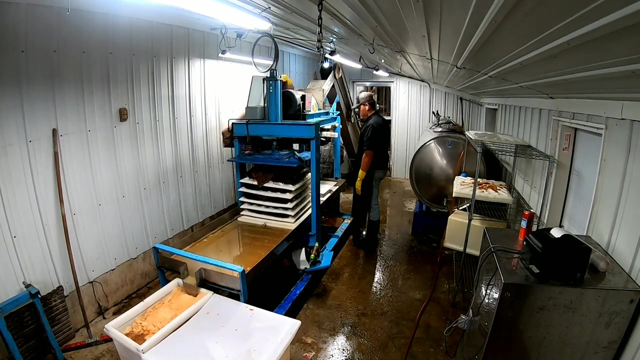 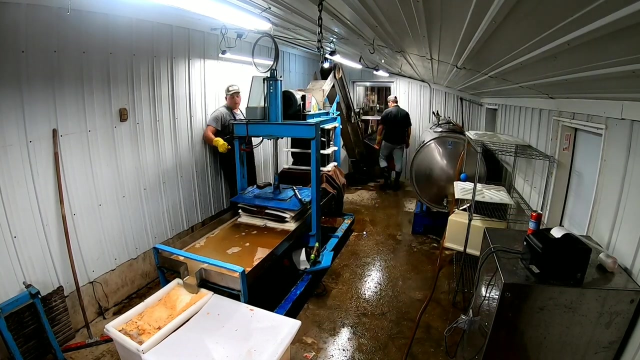 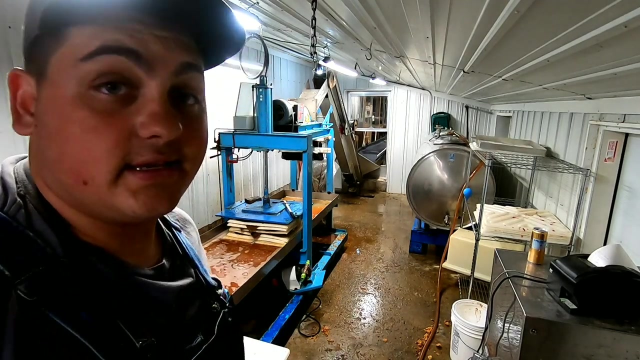 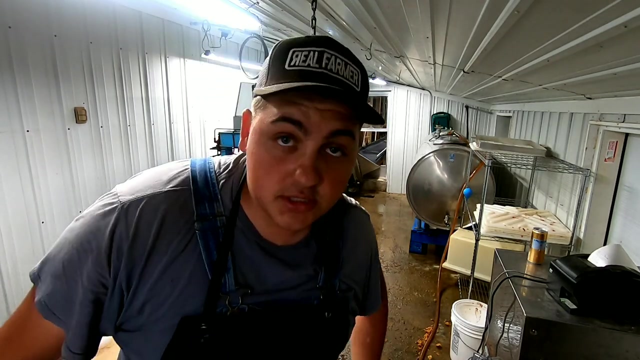 That should be good. You got the fancy, Fancy dandy red delicious here. Sure, works good, All right, All right, so this is the last press of the night, All right, so this is the last press of the night. it is late. it is currently 12: 40 am, so it's tuesday morning now we're still pressing cider. 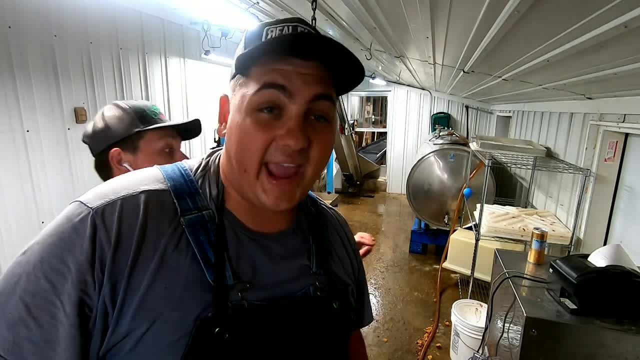 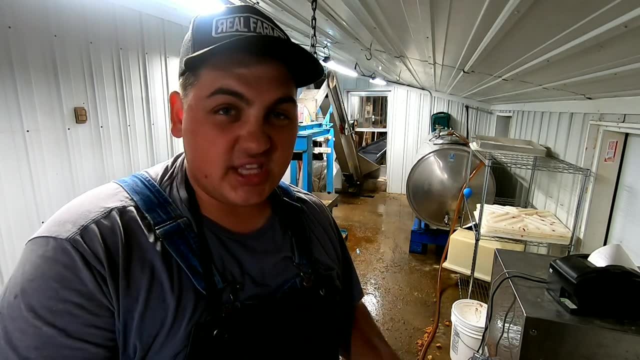 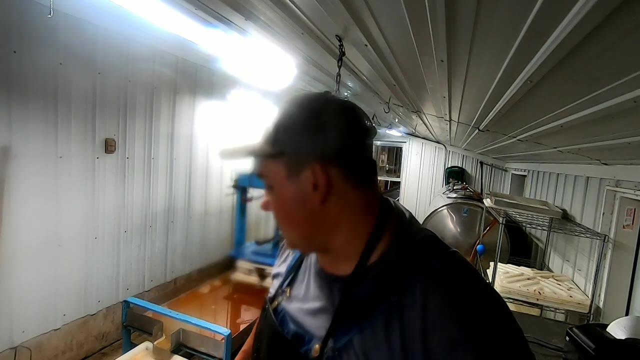 so our last bin was red delicious and it's a pain because red delicious this time of year they get. they get very, uh, soft, very mushy on the inside and the outside roll that real thick skin. as i was saying before my camera battery died, that red delicious has a really thick skin. the 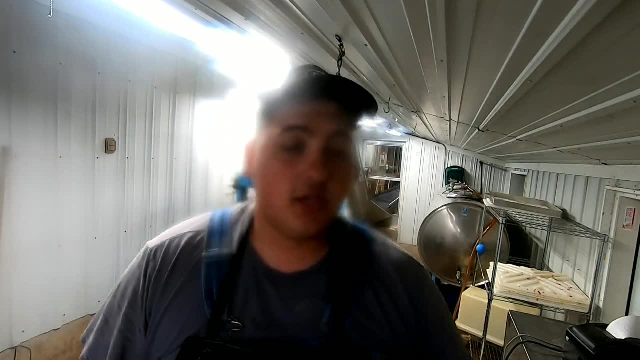 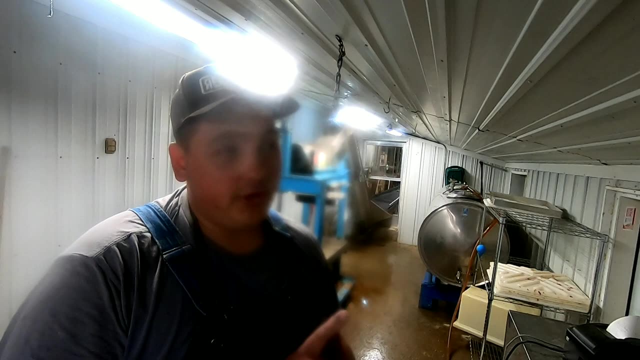 insides this time of year gets really mushy and really slimy so you can only put just a little bit inside the press there. so it takes a lot longer to uh, to press the bin. i know on the fujis and jonathan's on the fujis it takes about three presses per bin. that's the. that's the. 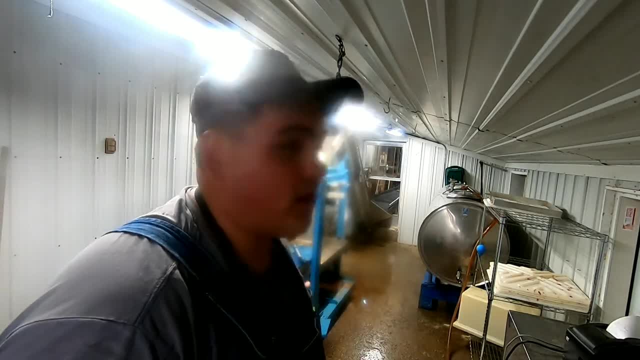 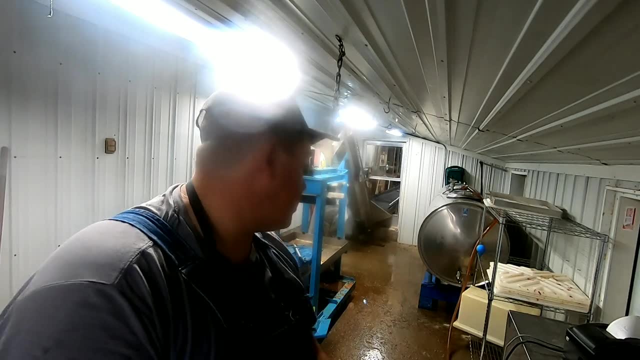 fastest. we ever pressed jonathan's between four and five, but on these red delicious probably eight or nine presses per bin, which takes you forever, because it's the same amount of work where you're doing less apples. so anyways, that's how we like doing the red delicious last, just because it takes a lot longer to tell. 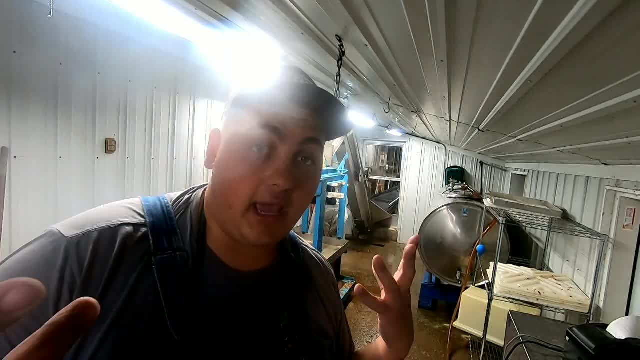 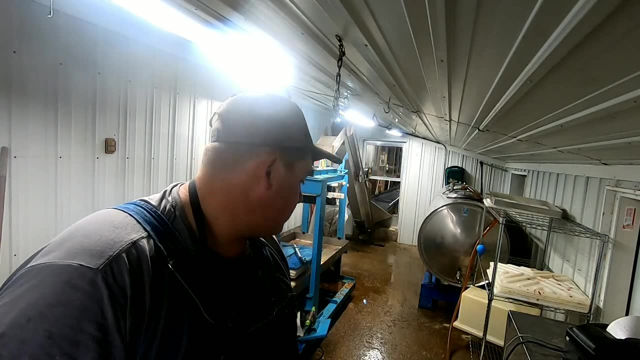 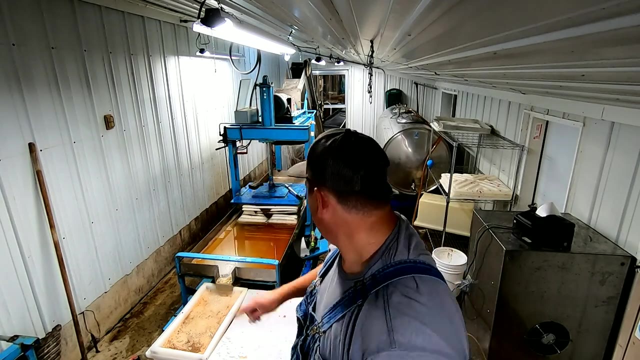 the time. but yeah, it's 12: 40 am and we just got done. now it's time to clean up this sloppy of a mess that's over here now, so that's always fun. so now that we are done pressing cider, we gotta wait for the pasteurizer. put all the cider through. the thing does its job. 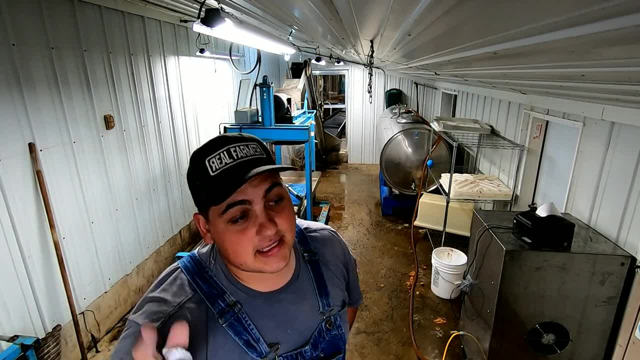 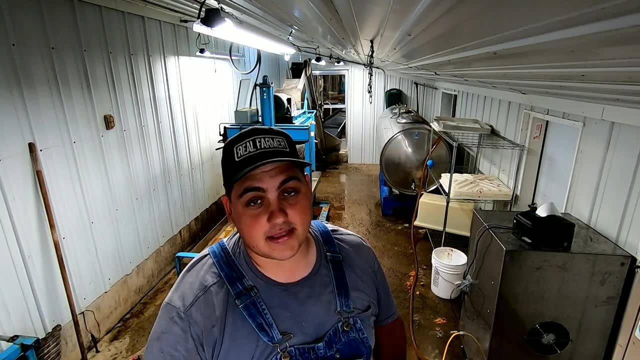 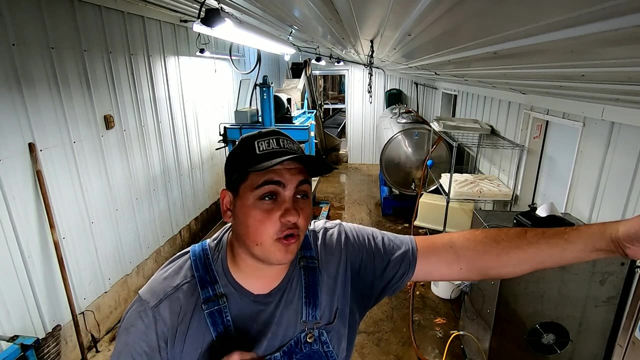 and then i'm gonna go ahead and start cleaning. but you guys are watching current day footage. i'm gonna be editing it tonight and uploading it tomorrow. i got a quick question for you guys: what time is the best to upload? for you guys, what's the most convenient time? is it in the morning, in the afternoon, and if it is like 4, 5, 6? 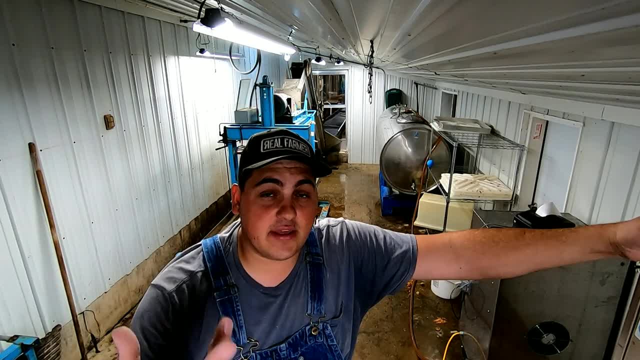 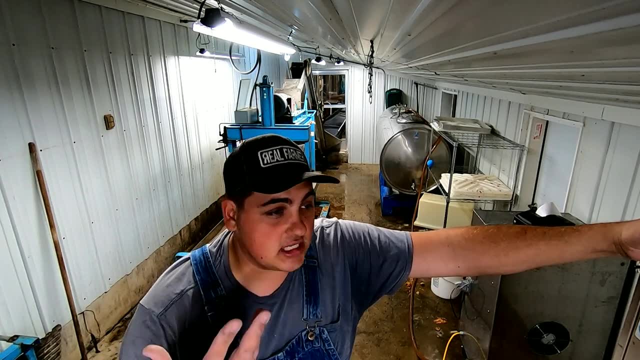 o'clock. let me know, because i want to start uploading consistently at the same time. just that just helps out with the whole entire youtube thing. so let me know what time of the day is the best for you guys. let me know if you're watching this video at 6 or 7 in the morning, 6 o'clock, let. 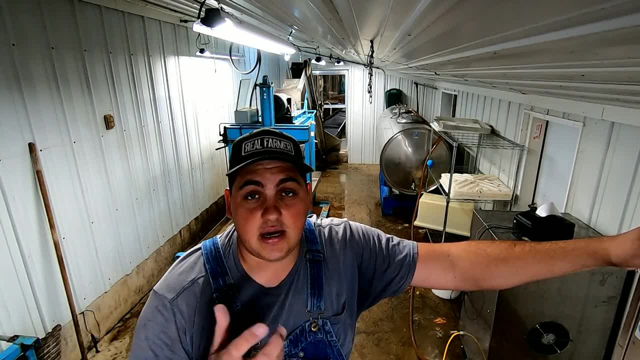 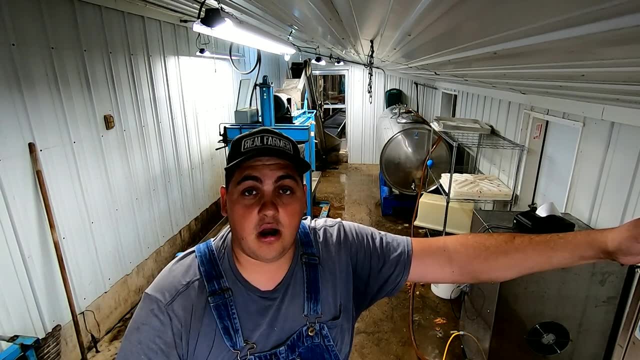 me know, because i want to start uploading consistently at the same time. just that just helps. is, uh, most available, most convenient for you, for you guys, and then i'm gonna get the um the most common hour, and then i'm just gonna start uploading it. that's consistent time, every single day. 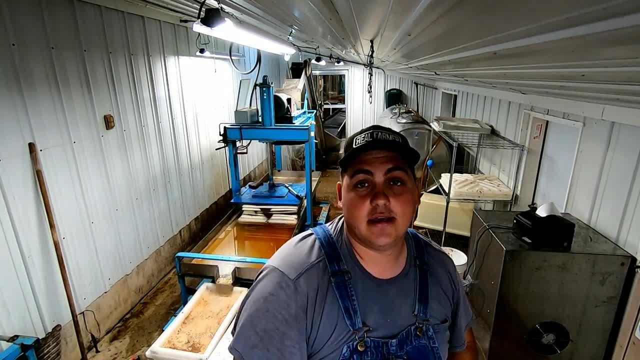 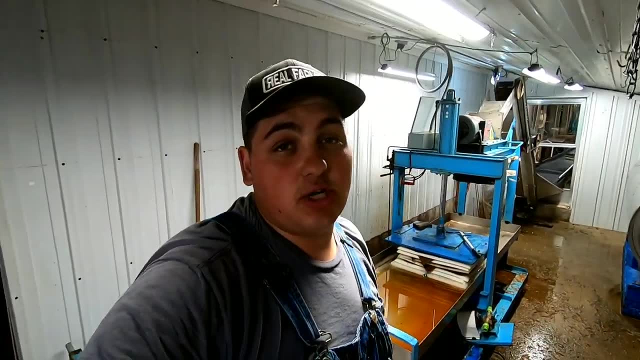 hopefully it works out. if not, i'll just keep doing, uh, doing it whenever it uploads. hey, all righty. so now that i'm waiting until this pasteurizer gets done here, i want to talk to you guys a little bit about the difference between apple cider and apple juice. i know there's some confusion there, a lot of. 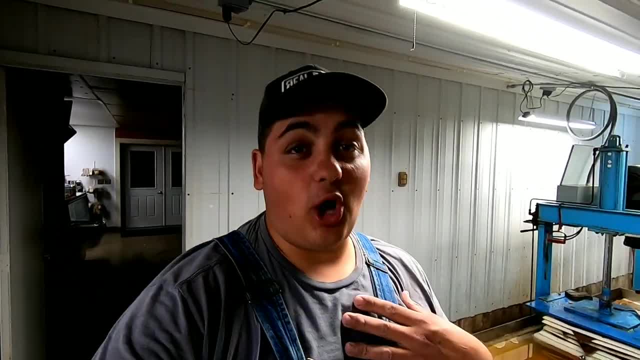 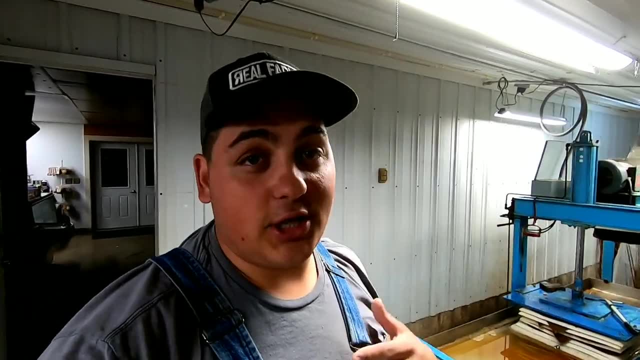 people think it's the same thing, but it's actually not the same thing and this is all based on my opinion here. there is no scientific fact. i guess, if you google, i'm not even gonna google. i'm just gonna tell you guys what i believe in. as an apple farmer and as a guy who makes apple cider, i'm gonna. 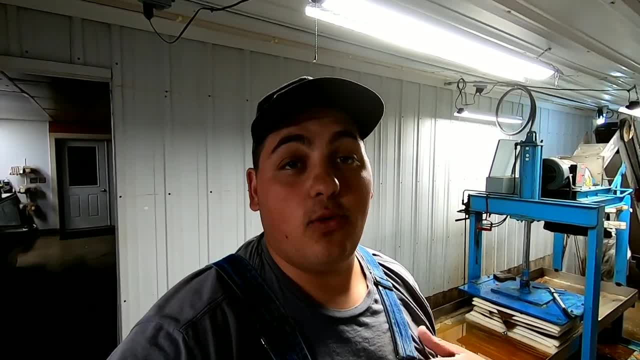 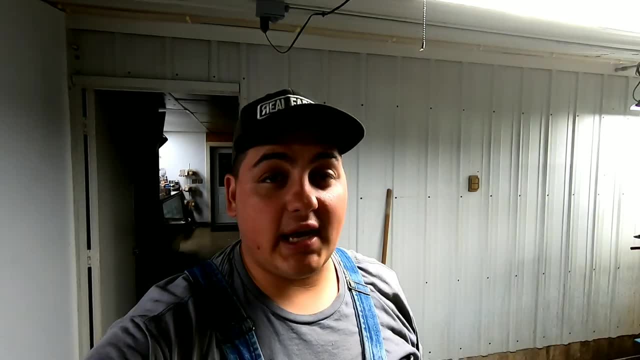 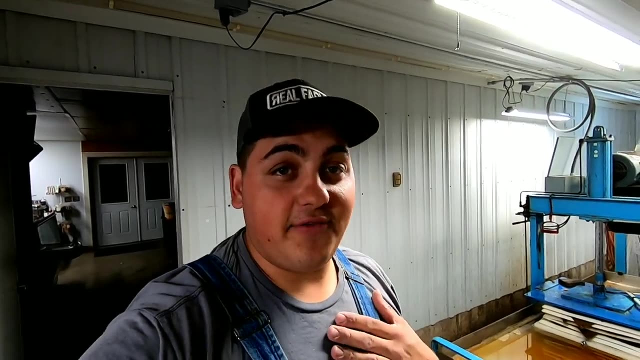 tell you guys what my opinion of apple cider is and what, in my opinion, apple juice is. so, as a apple farmer and the person who makes cider, apple cider is just ground up apples and pressed and then pumped into a tank and then you go ahead and bottle it up. so that's my definition of apple cider. whenever it comes to 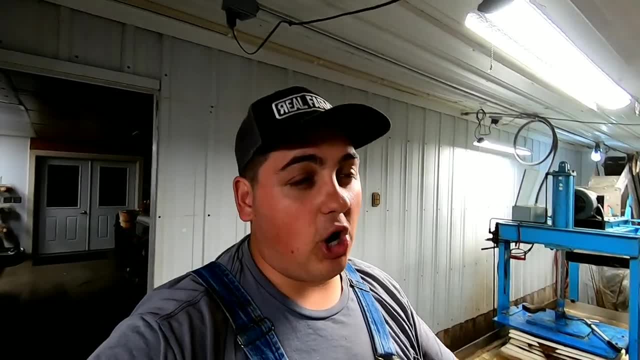 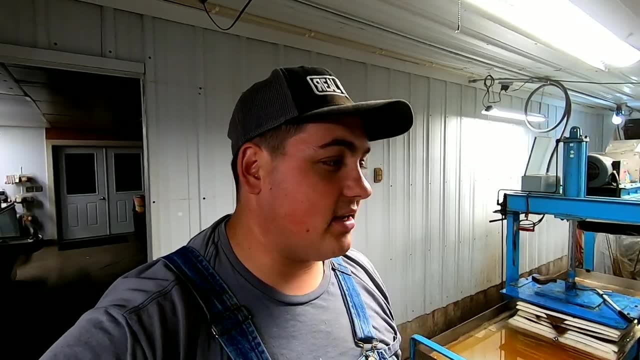 apple juice. i always think about apple juice in like small containers and cartons, the stuff i grew up drinking in school, and that stuff is processed, it's filtered. i mean it has all kinds of stuff added to it: preservatives, have sugar added to it, has water added to it. so the biggest thing i tell 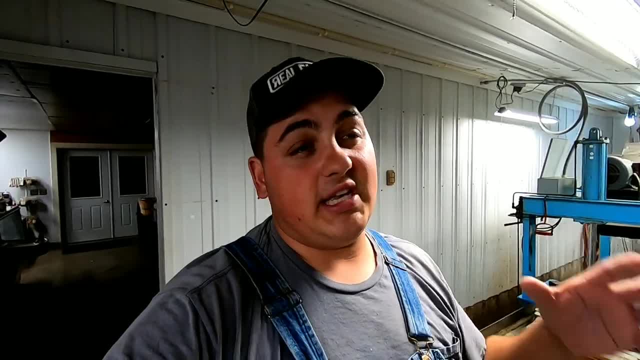 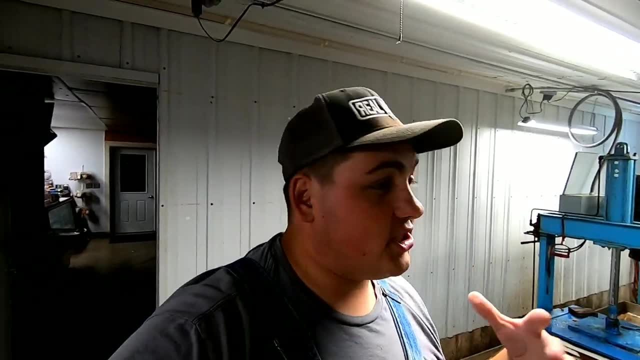 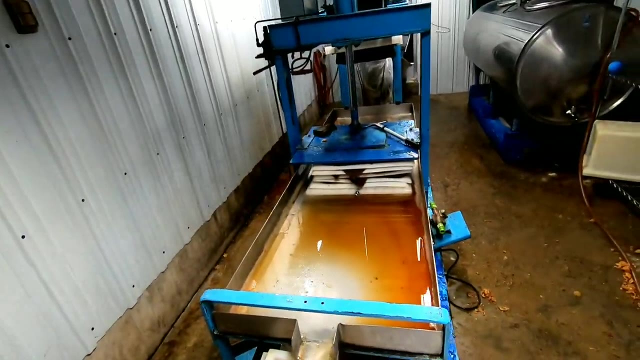 all the field trip groups that come out to the farm, i tell them apple juice is processed and apple cider is a raw juice that comes straight from the apples. so i mean, this is just a farmer's definition of the difference, but that's, that's how it is to this. you see here, this is apple cider, where we're. 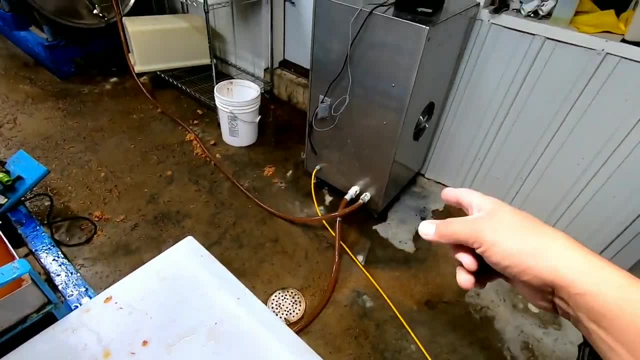 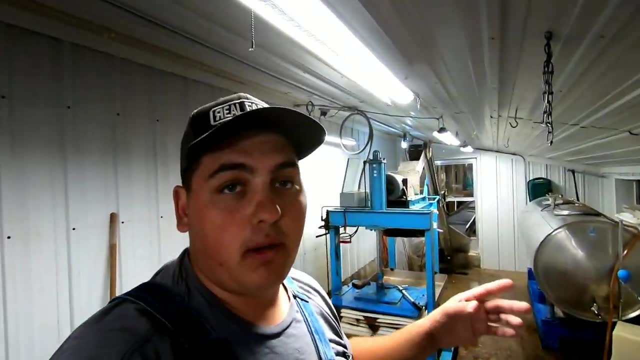 selling here. so the apples are grinded, pressed and then we have to uv pasteurize our cider just because the whole health department thing- the health department would not, wouldn't allow us to sell our cider if it's not pasteurized- and all ciders and juices in the united states. 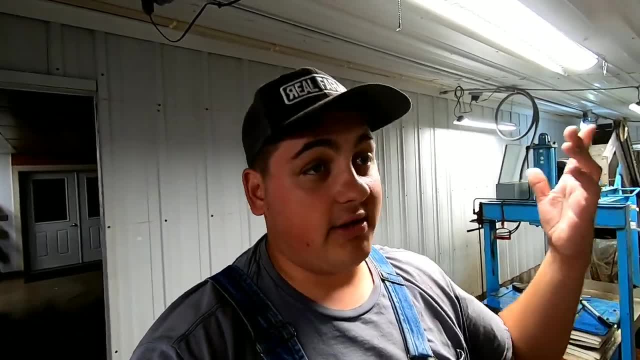 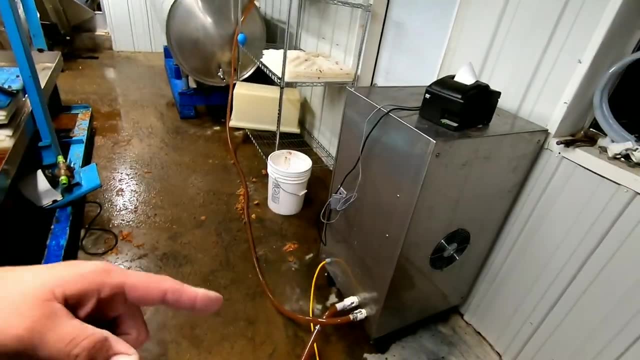 have to be this way. unless you cannot commercially sell your cider, you're not gonna sell it and you're not gonna sell it or it can't even sell it at a farmer's market, just because all the food safety reasons and stuff like that. but all we do is uv pasteurize it. it just kills off the instant bacteria, the 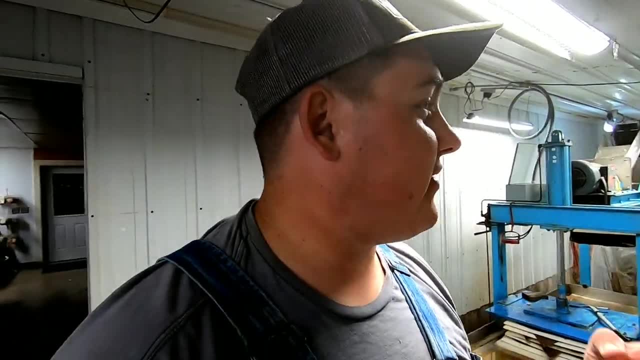 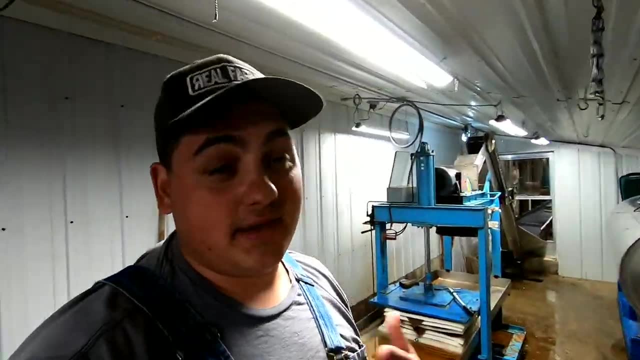 benefit of the uv pasteurizer: it doesn't break down the pectin, so you still have that nice fresh flavor of the cider. we pump it into the tank and then we just bottle it and that to me, that is apple cider. apple juice, like i said, is processed. they have stuff to it, they take stuff out of it.